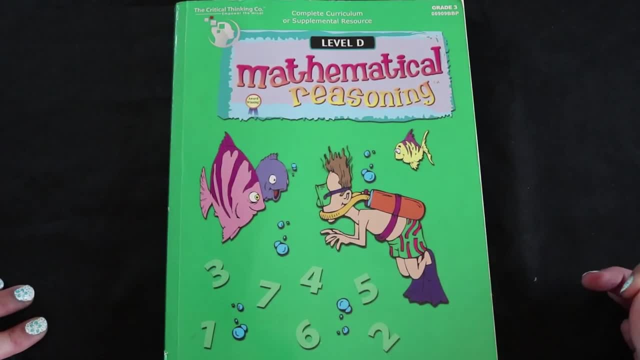 It didn't have anything wrong with it. It was just like a buyer's return copy. So I highly suggest checking out the Amazon Marketplace or Amazon Marketplacecom to learn more about it. We also have other online sites for used, like new curriculum, to help save some money. Just. 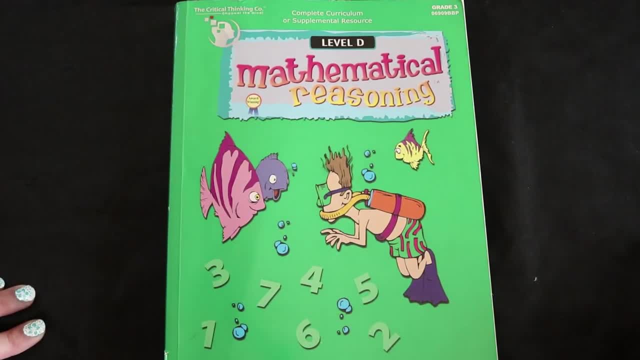 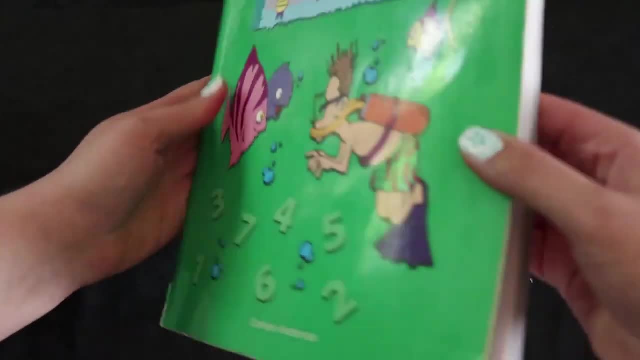 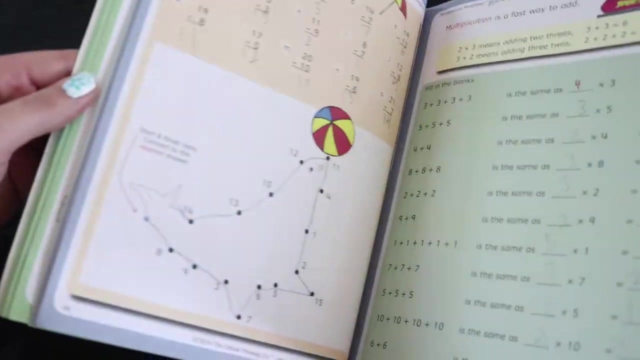 for the price alone if you can find cheaper like new copies. I think this is a really nicely done full math curriculum. These color sections you see here on the edges don't mean anything. That's just to add to the color. So there's not like chapters or sections to. 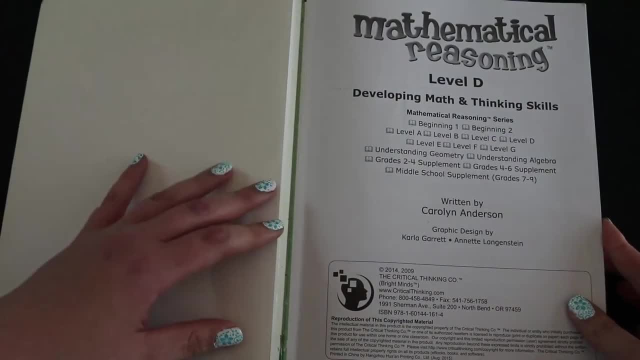 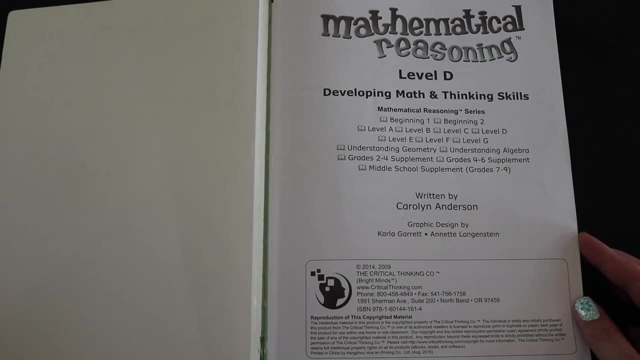 follow. We just started at the beginning and had been doing just four pages a day. We're just rewriting it from ninth to eight But we cut it down to two pages when we got our Math Mammoth curriculum. We had a rocky start for our first year and couldn't get any curriculum. 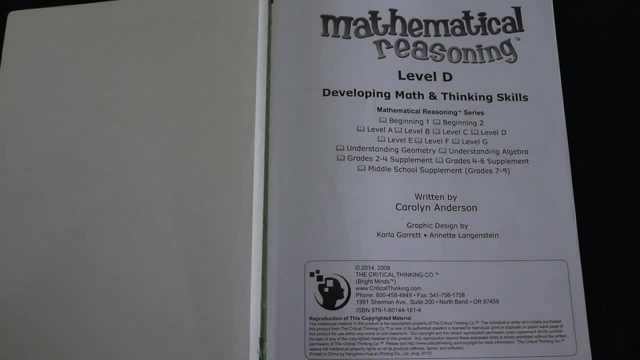 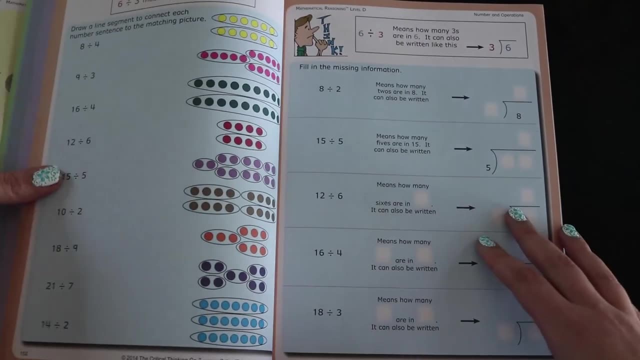 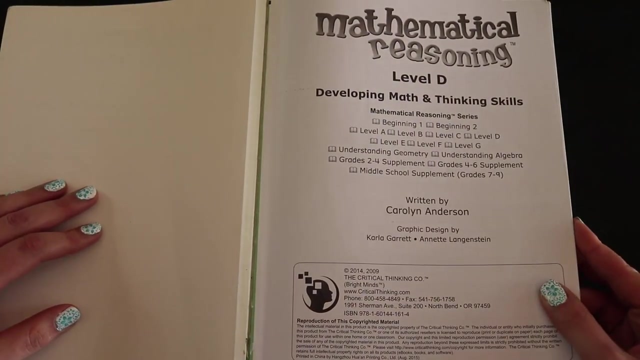 we wanted to use until the beginning in 2018, which was halfway through our year, because we started in July 2018, so that's why she's on page 152.. We're barely halfway through the book, But that's not a big deal, because we homeschool hear and way and we'll just continue working through it after thing week. That's why I think that's a nice pack, But you'll have to do a good job on it. And then the big thing with math formation included is that 어제 I finished a newlove раз. 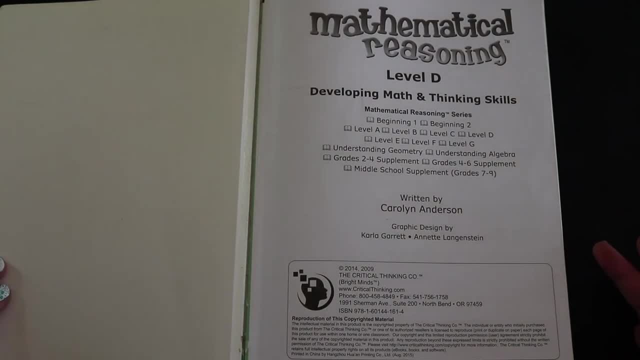 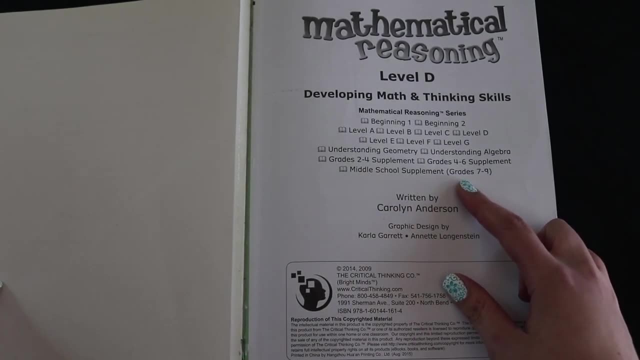 summer break and into her fourth grade year. That also just gives me time to save up for level E, So we plan to use this curriculum all the way as far as we can for both of my girls. They have beginnings one and two for pre-K levels, and then level A is grade. 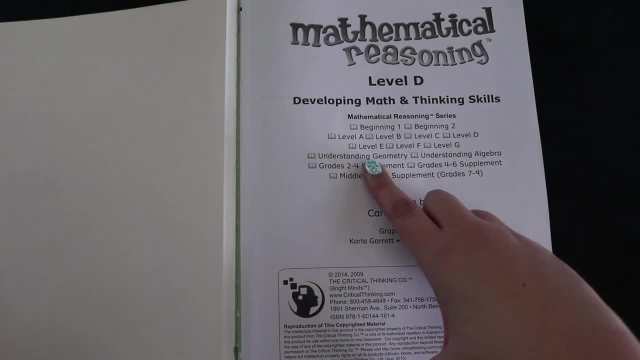 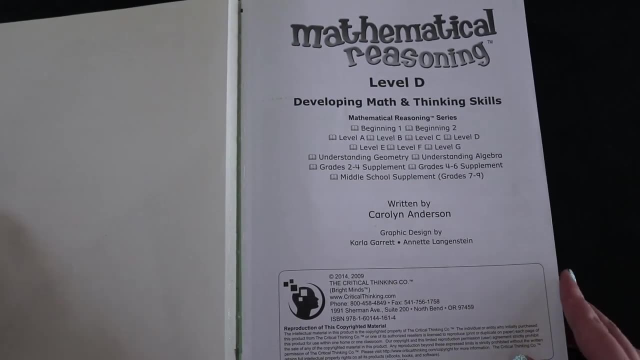 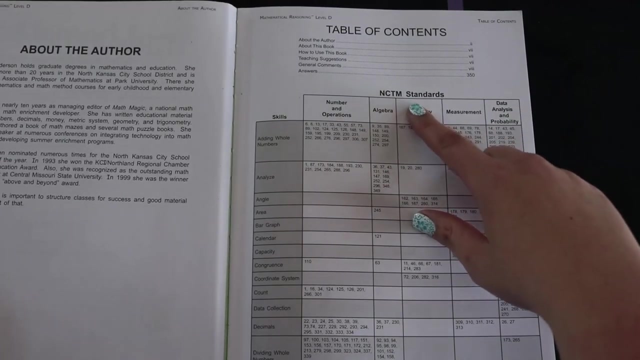 one and up to level G for grade six, Then for seventh through ninth grade they have understanding geometry algebra. they have different supplements and they also have an understanding pre-algebra, one which isn't listed there. Mathematical reasoning uses the NCTM standards. I'll have a link to explain more about those down in the description box. 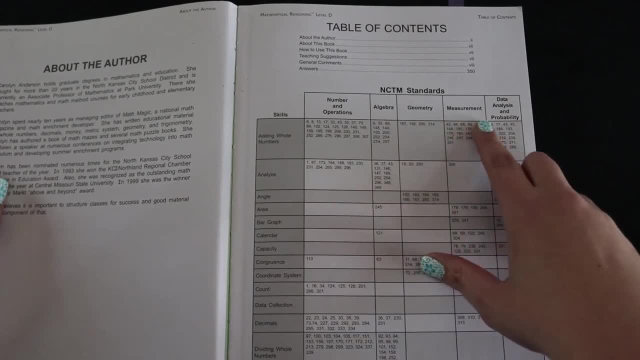 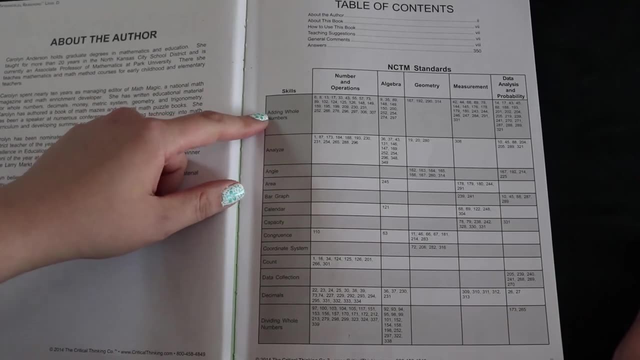 The standards pretty much are numbers and operations, algebra, geometry, measurement, data analysis and probability. And for level D they go through a whole ton of skills from adding whole numbers, analyze angles, area bar, graph, calendar and so on, And then they 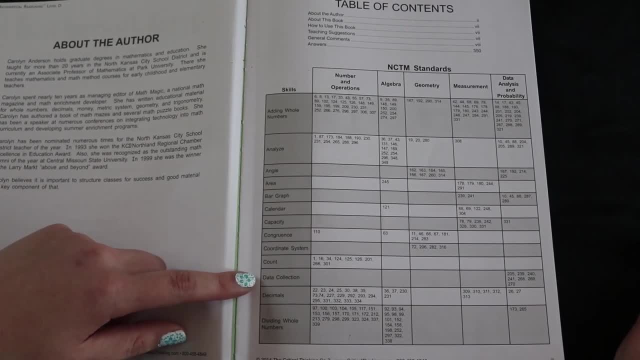 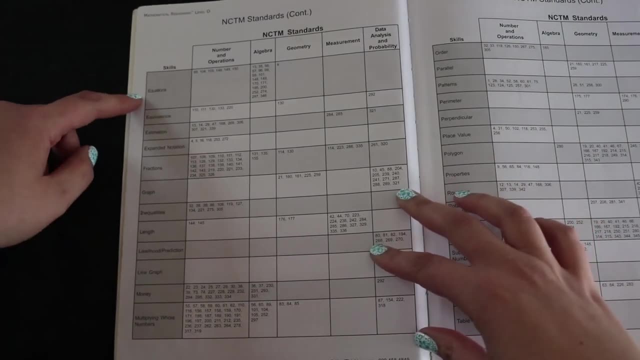 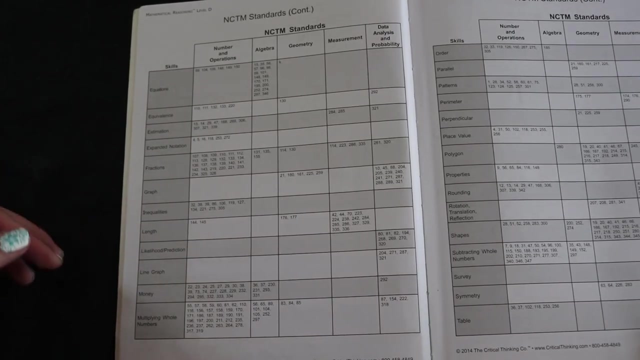 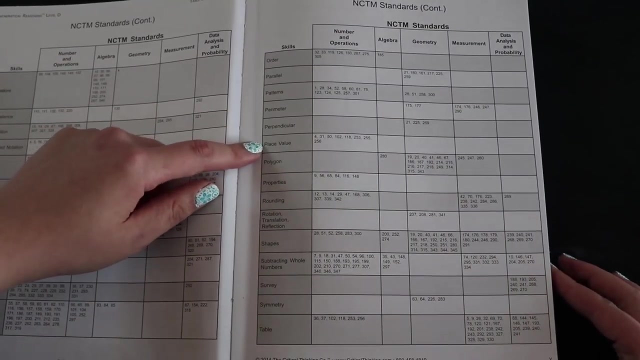 compare capacity, congruence, coordinate system, count data collection, decimals dividing whole numbers, equations, equivalence estimation, expanded notation, fractions graph inequalities, length, likelihood and prediction line graph. money multiplying whole numbers: order, parallels, patterns, perimeter, perpendicular place values, polygons. 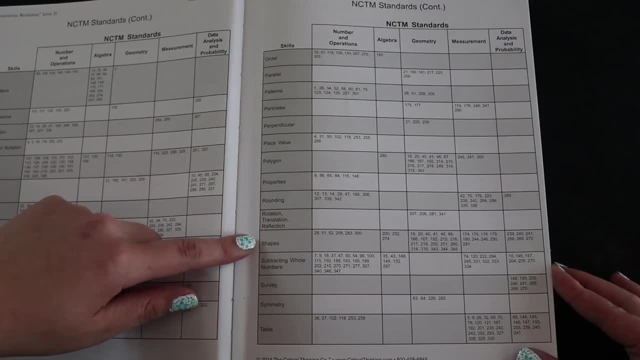 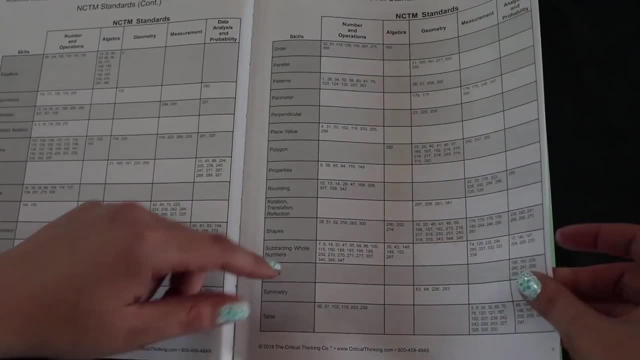 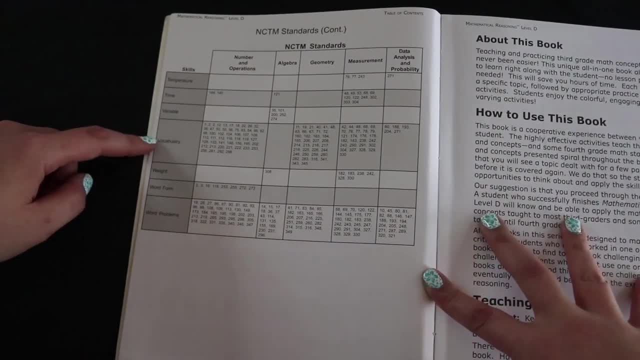 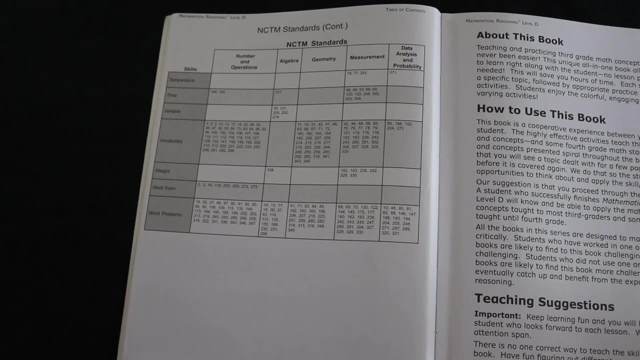 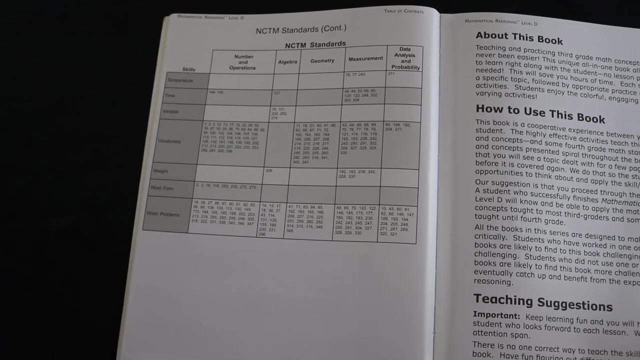 vocabulary, weight, word form and word problems. And then, should you want to use this as supplemental resource, they list page numbers for each of these skills and what operations or standards rather that they go under. So, should you want to jump around instead of, 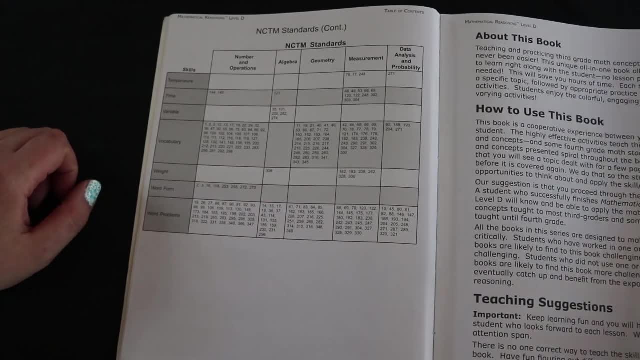 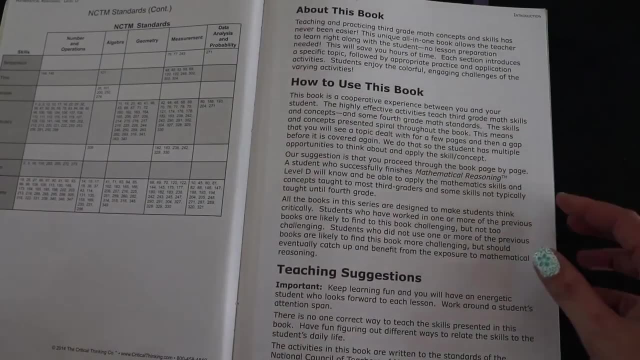 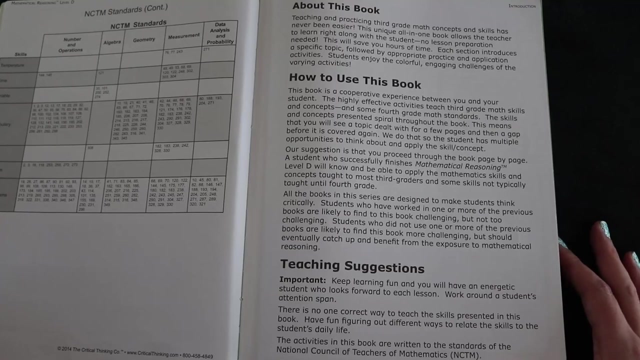 word, page by page. that'd be extremely helpful. Over here it talks about the book, how to use it and teaching suggestions. It takes a spiral approach throughout the book, meaning it introduced and covered a topic for a few pages and then a gap before it covers again. 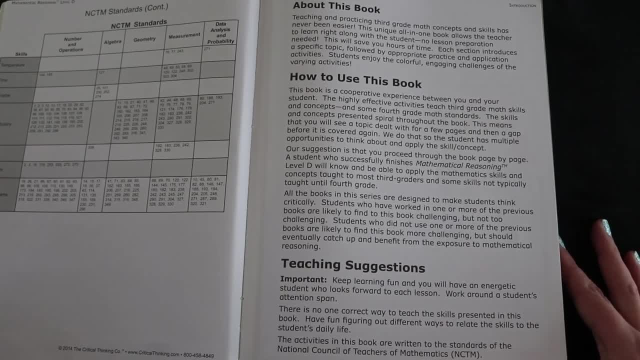 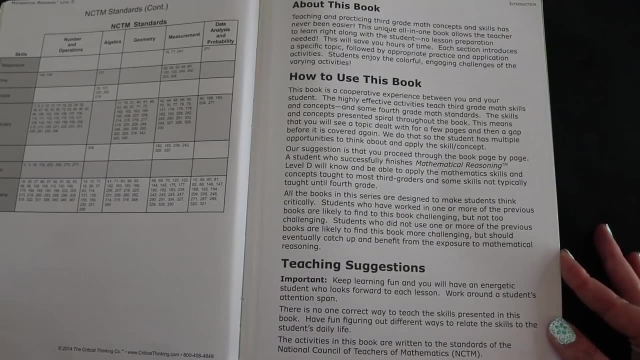 They do that so that students have multiple opportunities to apply the scalar concept. They suggest working page by page and they also mention that students that have worked in previous mathematical reasoning books are likely to find this level challenging, but not too challenging, and for students just jumping right in without previous exposure. 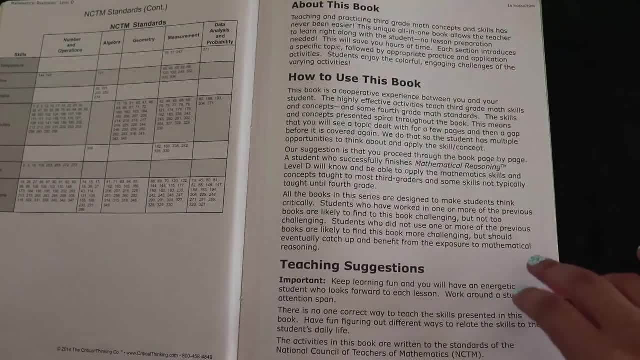 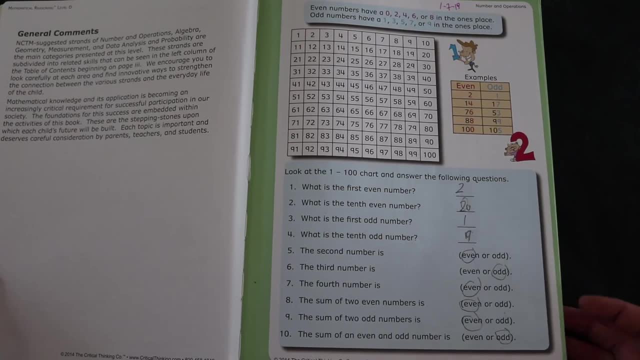 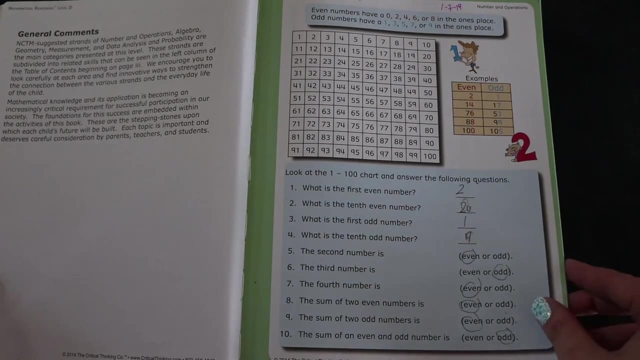 will find it challenging, they'll be able to catch up and benefit from using this book anyway. Starting at the beginning are simpler number and operation skills, which will tell you which standard they're working on in the upper right corner. They start out simple to ease kids into everything using easier, probably more well-known skills. 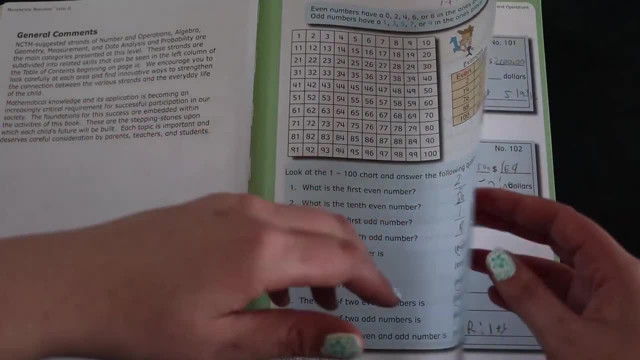 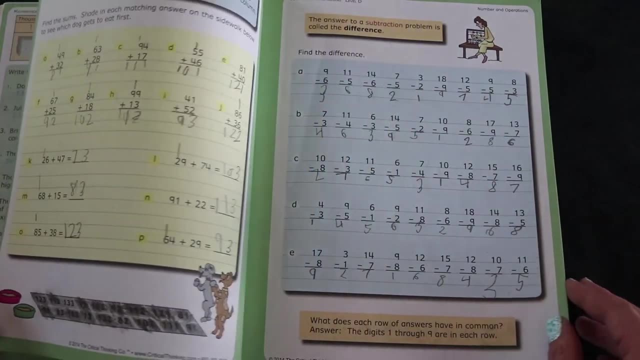 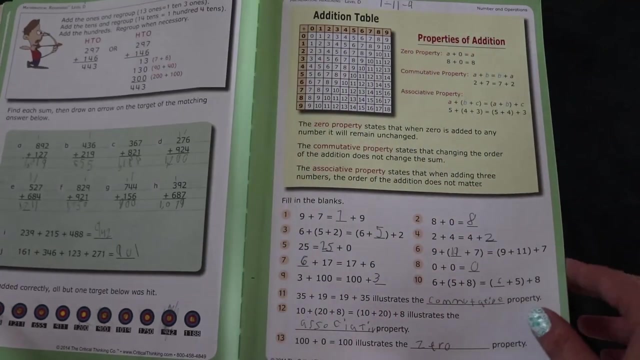 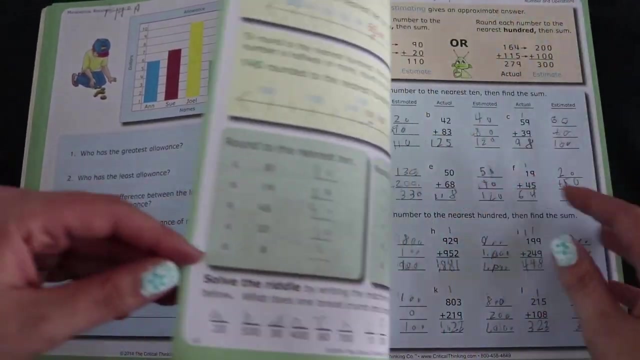 each page is full-color and the content is rather large, but the lessons are short, so it doesn't look like a ton of overwhelming work to do. Most pages are different, with a few scattered similar activities, but that really helps avoiding monotony that some other math curriculums have. 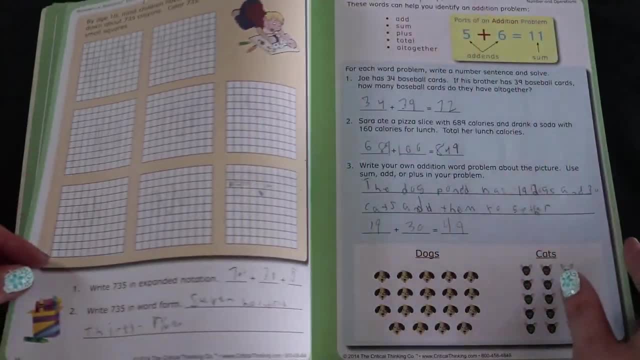 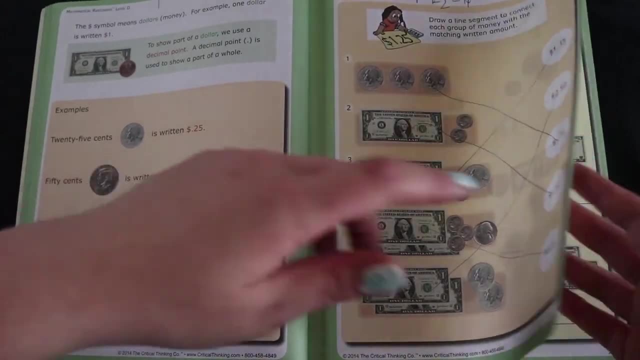 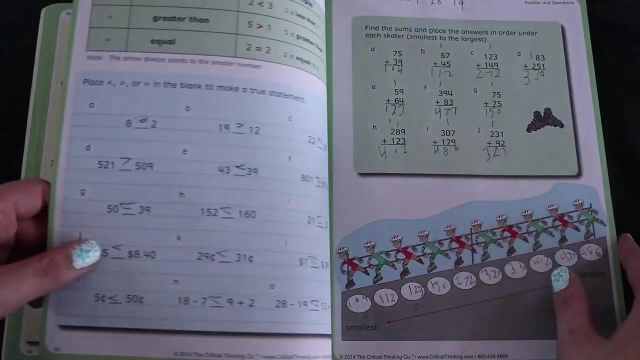 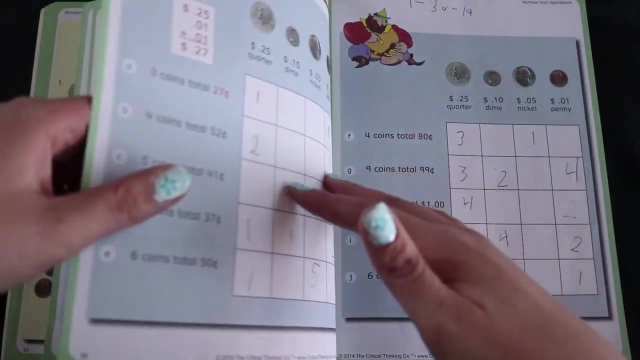 It doesn't take very long to introduce new topics. So here's still numbers and operations, but then here's working on geometry and then right into money. Numbers and operations again, and here's algebra. I think it's really great that they start basic ideas and concepts in algebra early. 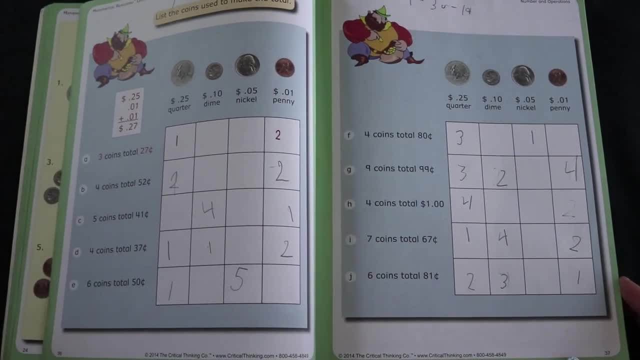 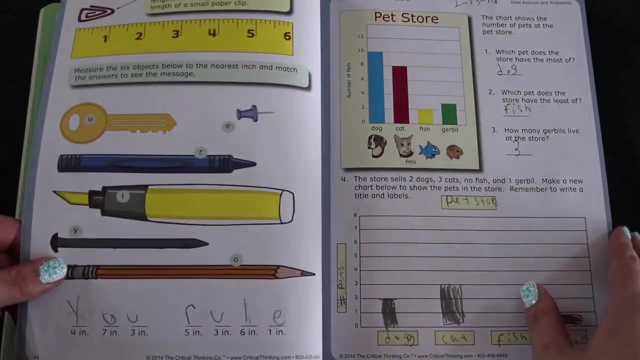 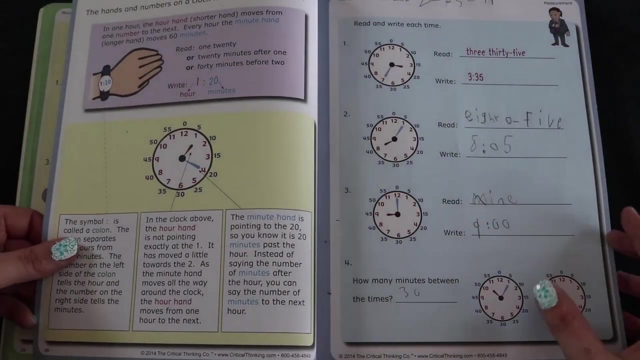 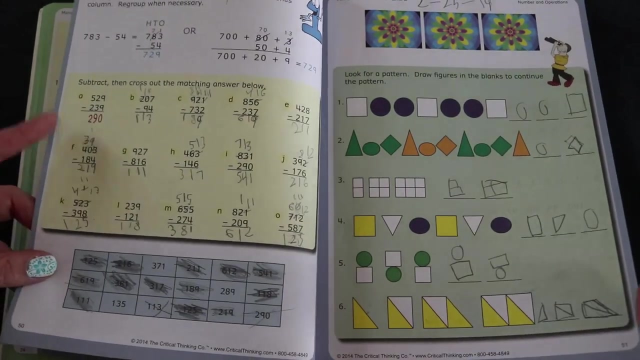 like this, because then it just gets them more comfortable for when they really get into it, like in the upper grades and middle school and such Measurement, data analysis and probability, more geometry, and then it gets into time. They got patterns doing three-digit subtraction and this is like when they come up with vocabulary. 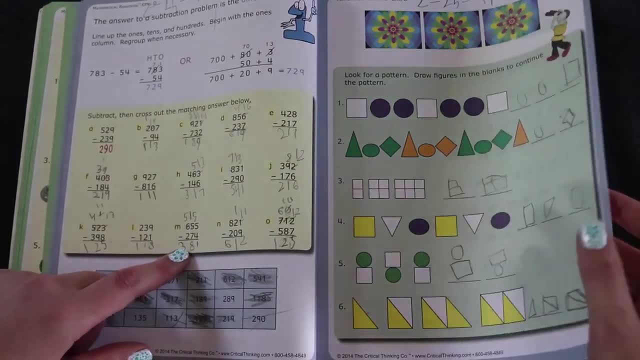 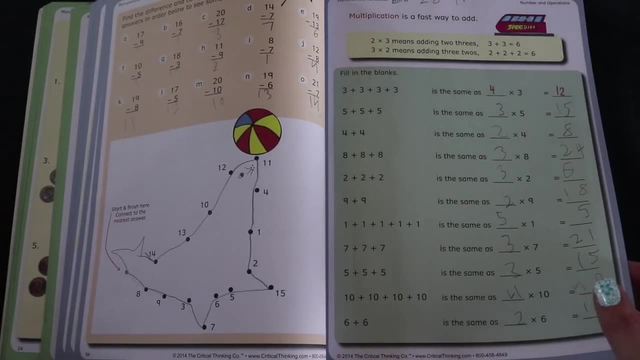 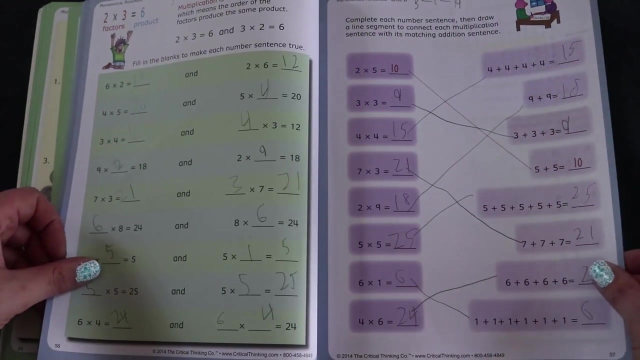 words. they're bolded in different colors and they give different. in some pages they give different words Like meanings, like subtraction, less than or like what is the difference, like those kind of words to help when they get into word problems and such. 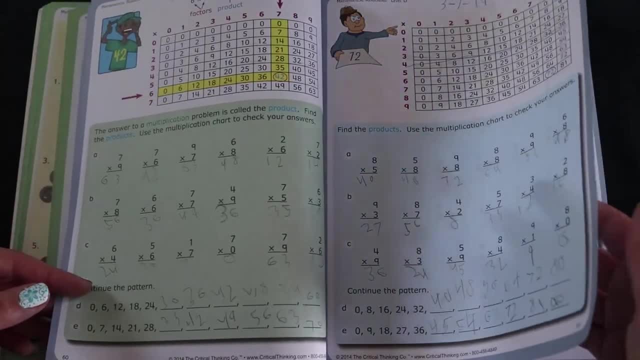 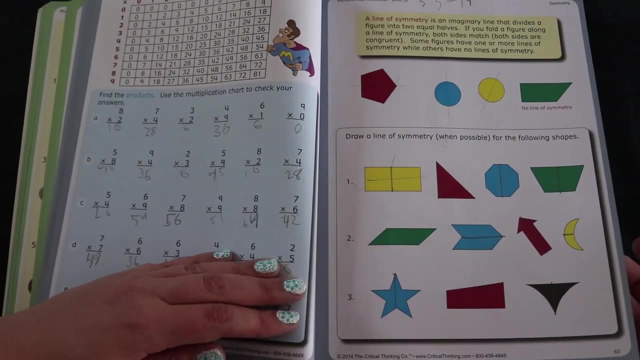 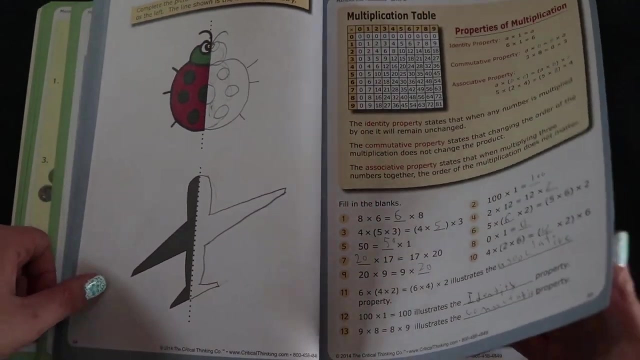 Here's multiplication. The instructions for each page are clear and easily understandable and, like I said, I like that it teaches the math vocabulary. My daughter works on this independently and when she's done I'll just look it over and make sure she's understood what she was working on. 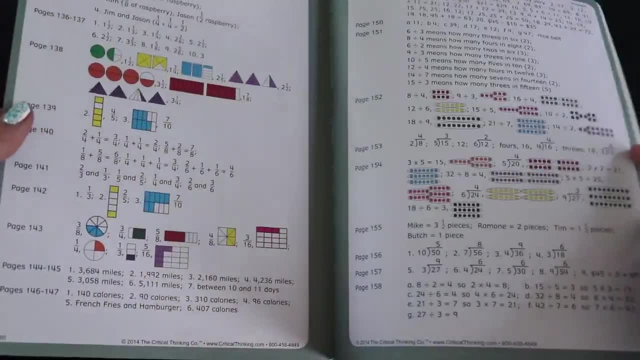 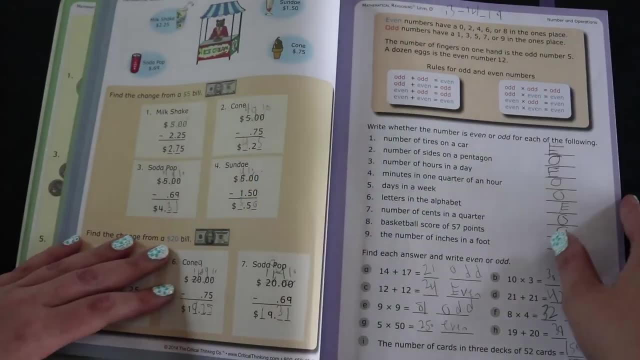 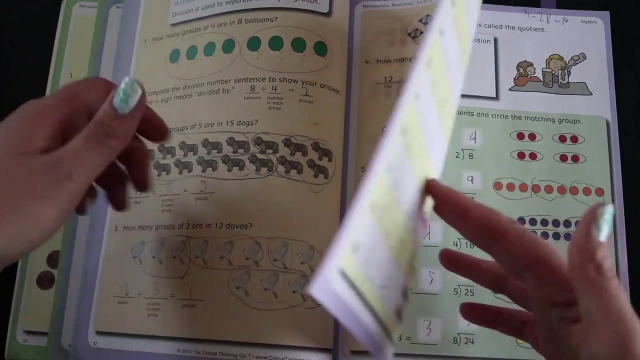 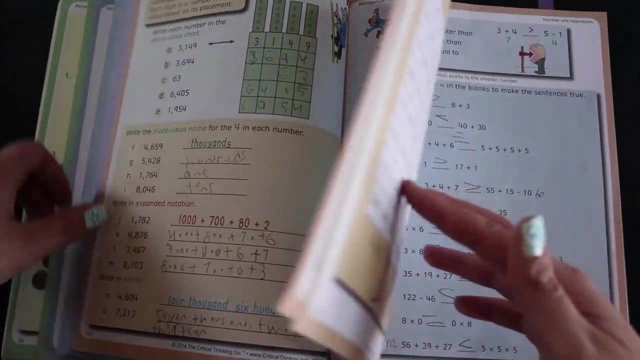 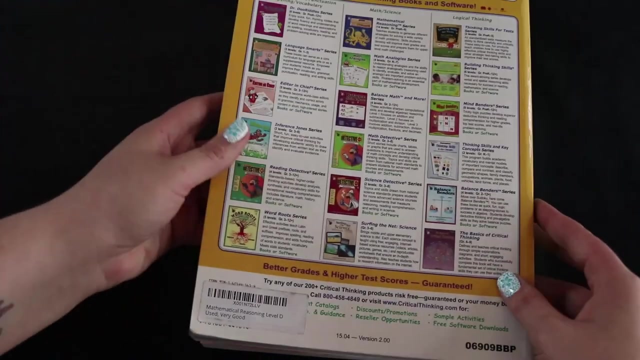 The back has full answer key if you don't want to sit there and correct everything yourself. so this is pretty helpful for me to save time. More measurement: They have different books that they have the critical thinking company. like these mind benders. 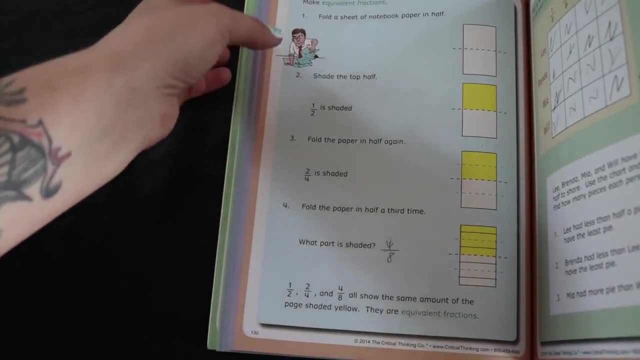 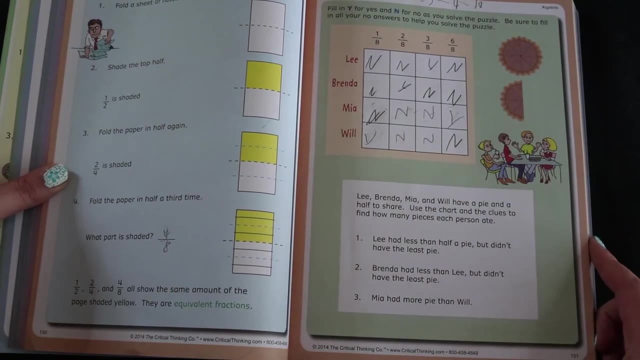 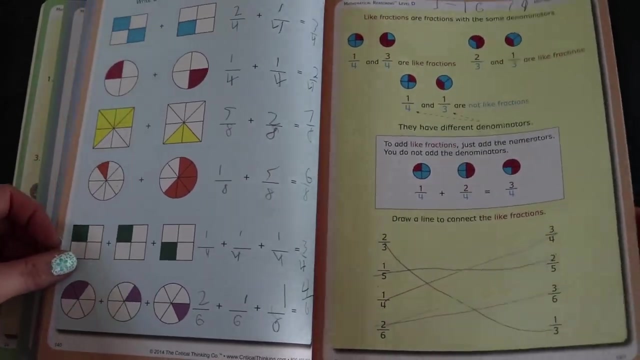 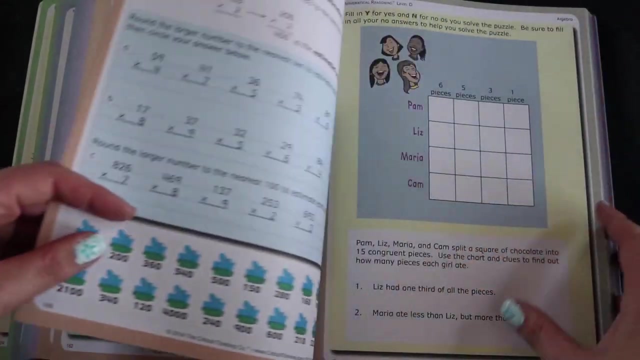 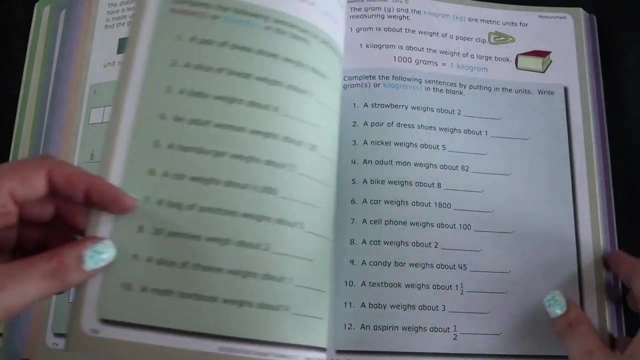 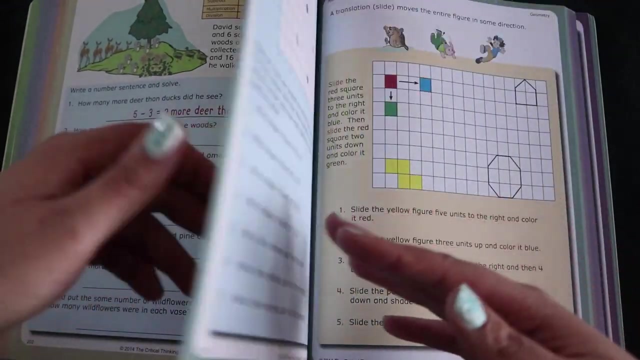 They have examples, not examples or samples, I guess also incorporated into this to help. Maybe if you wanted more activities like this, you could get separate books or workbooks to use for just thinking skills like that. Thank you, Here's plotting. 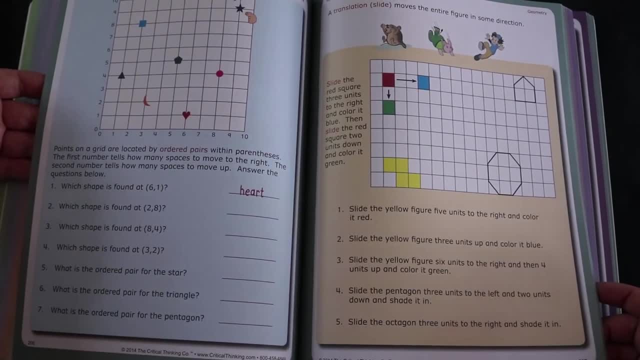 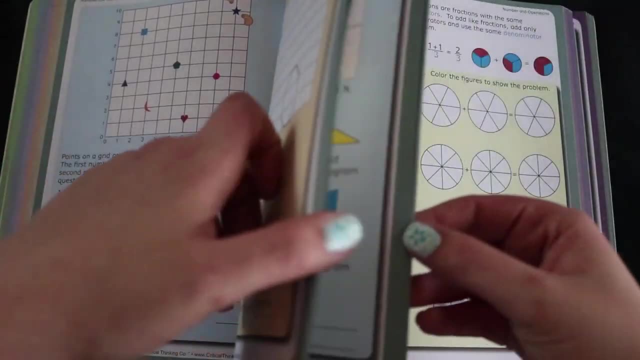 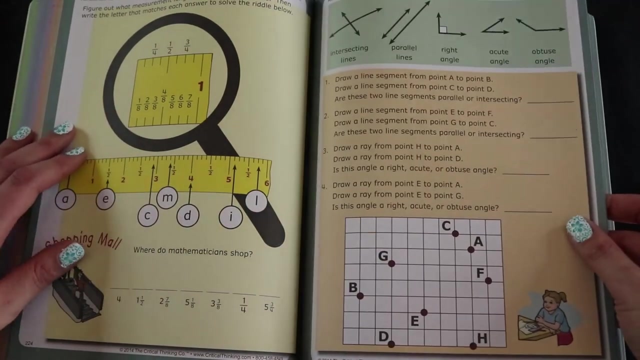 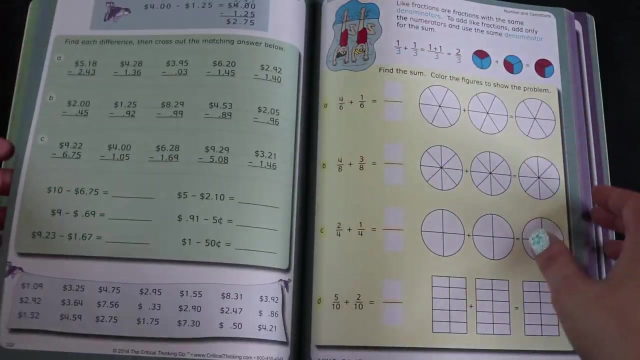 I don't remember doing this until like middle school, but this is third grade and they're already doing it, so it's pretty cool They start out with things like that on this level already: Intersecting lines, parallel lines, right angles, more plotting. 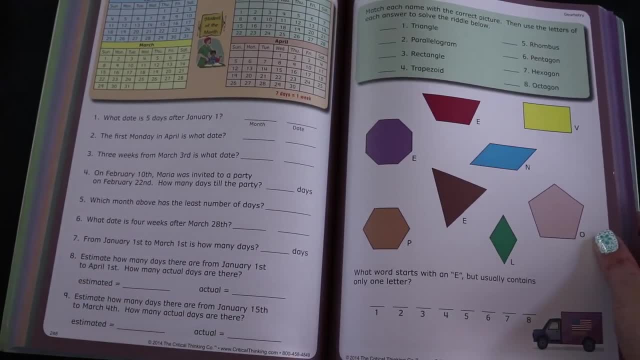 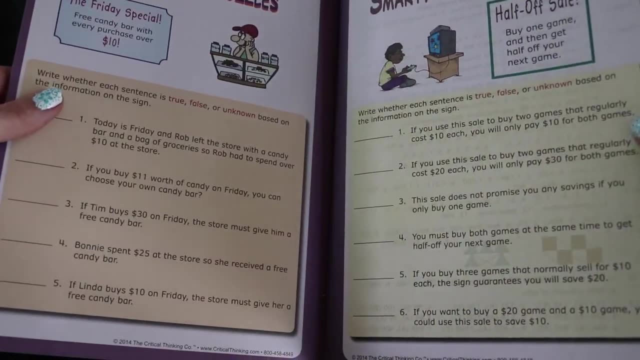 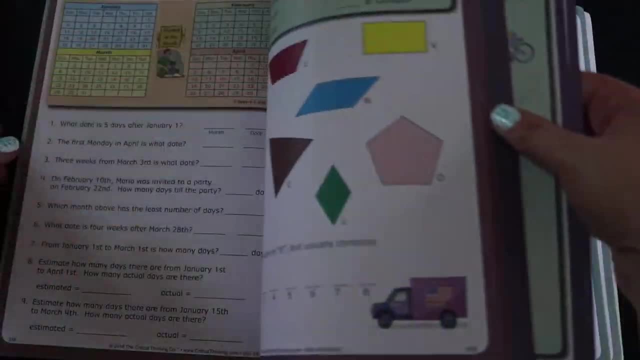 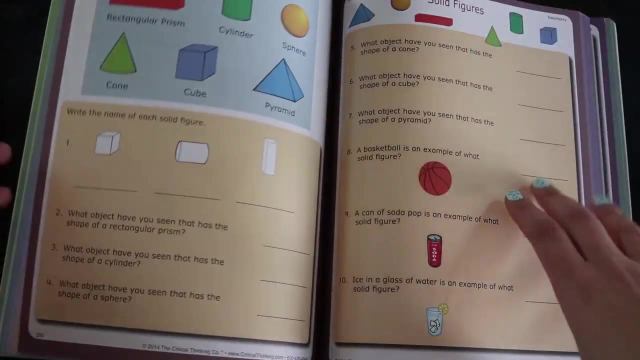 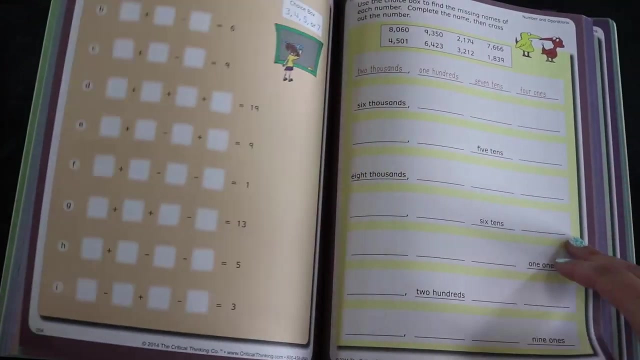 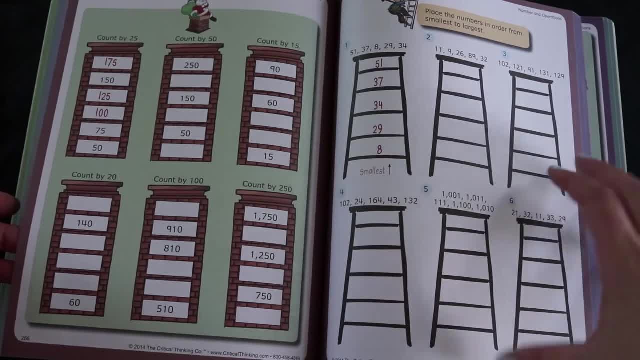 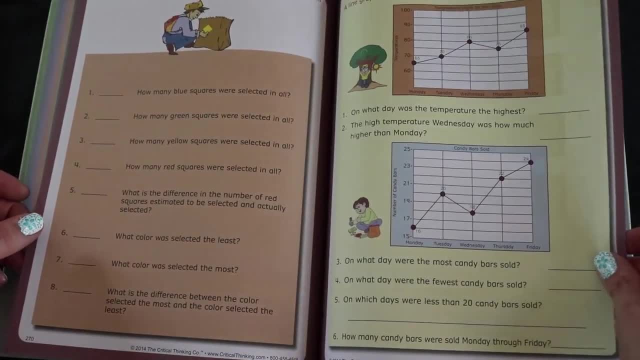 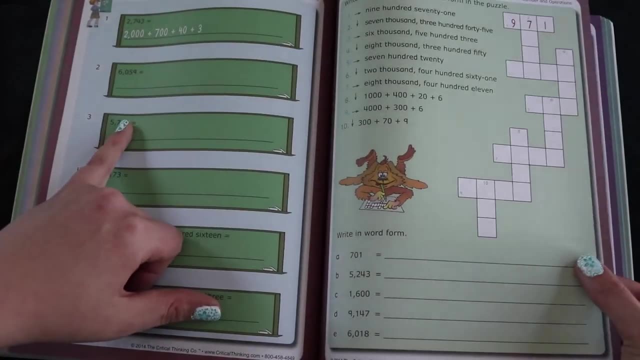 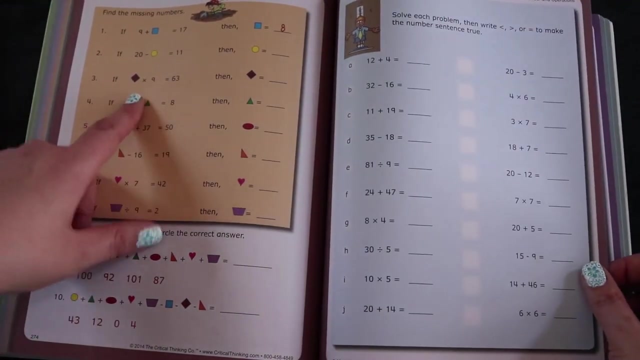 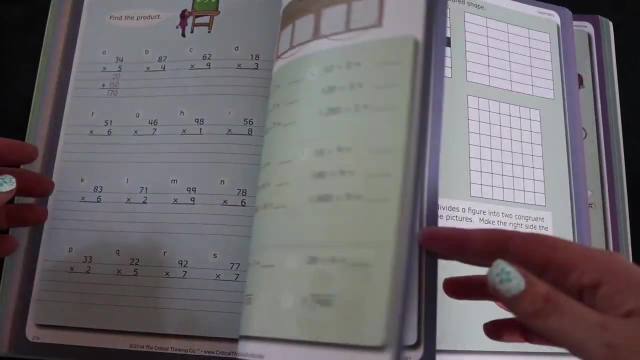 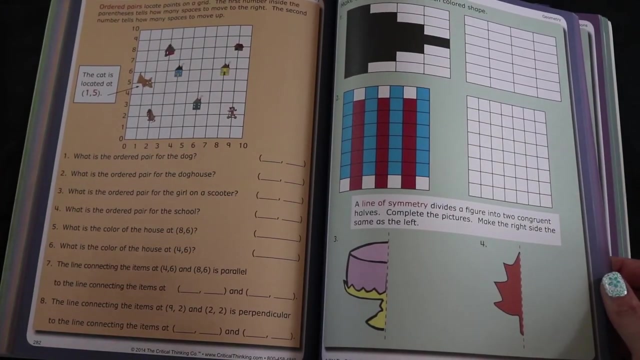 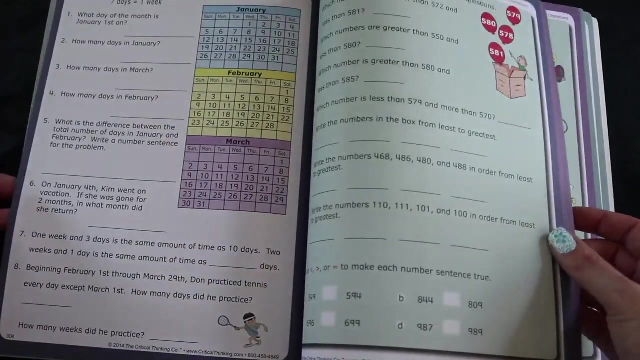 Patterns, Skip counting Links, counting to help those math facts it's great. graphs breaking numbers up into their place values, more algebra related stuff using symbols. yeah, just overall I think it's a pretty solid curriculum like it. there's so many topics and like in a clear, understanding way for the kids, it's not overwhelming. like I said,